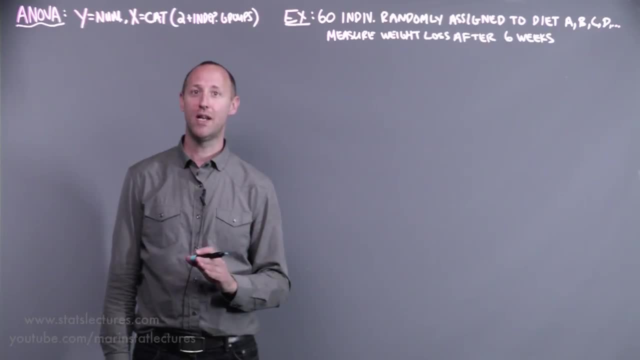 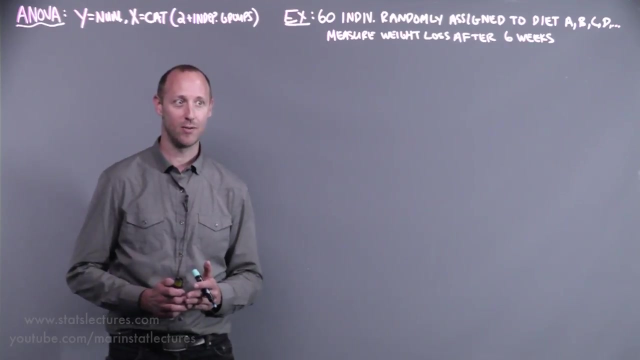 Analysis of variance in general is a concept that flows through many different statistical methods. So if you sit back and think about it, in some sense, analysis of variance or analyzing variability is- in some sense it could be another name for statistics. That's what this discipline is all about. 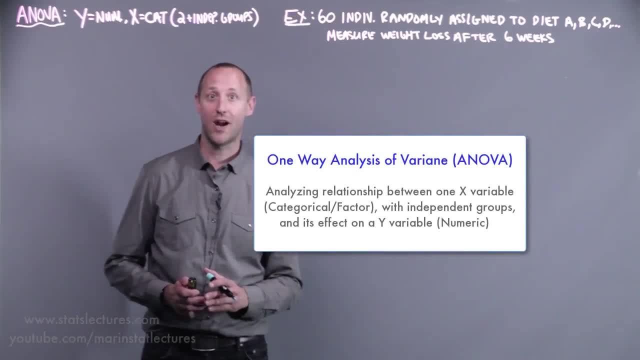 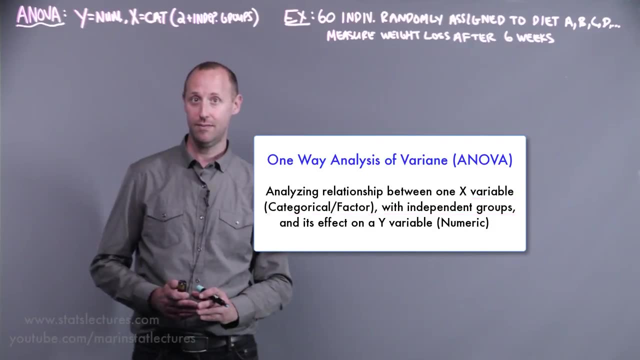 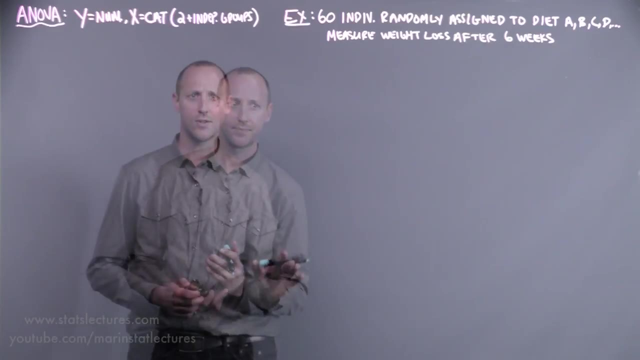 So this particular test, one-way analysis of variance- is for analyzing relationship between one x variable- that's categorical- with two or more independent levels or independent groups, and their effect on some y variable. that's numeric. Okay, some numeric outcome. So we're going to work with this simple data here. 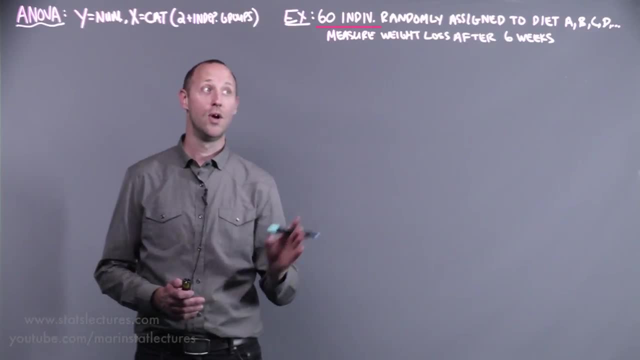 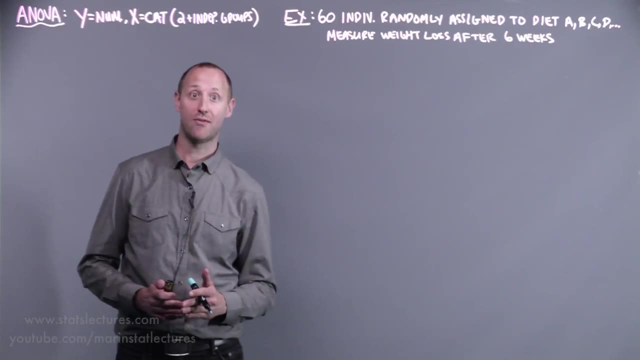 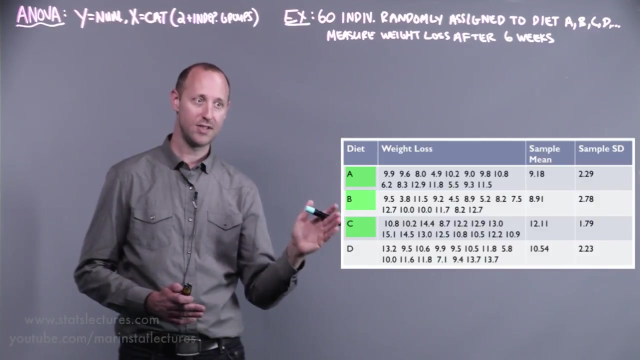 We can see we have 60 individuals who are randomly assigned to one of four diets. We're calling them diets A, B, C or D And they have their weight loss measured after six weeks of being on the diet. So we can see 15 people have been assigned to diet A, 15 to B, 15 to C and 15 to D. 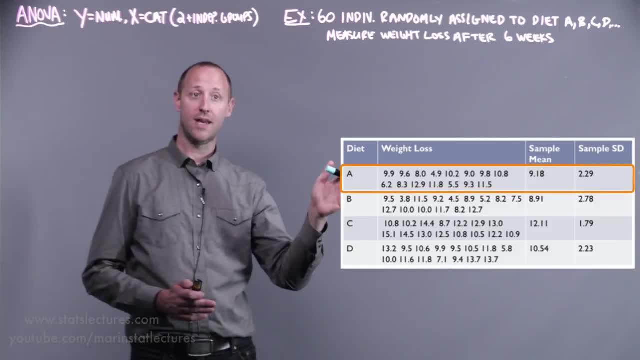 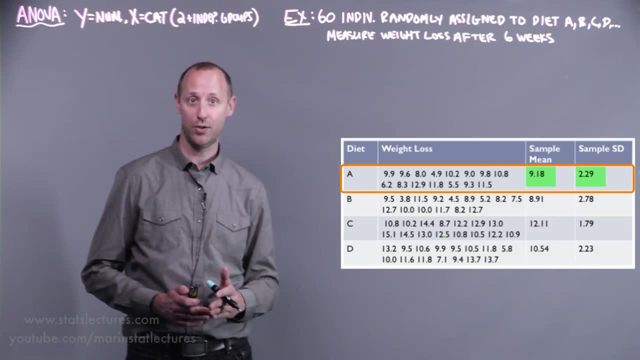 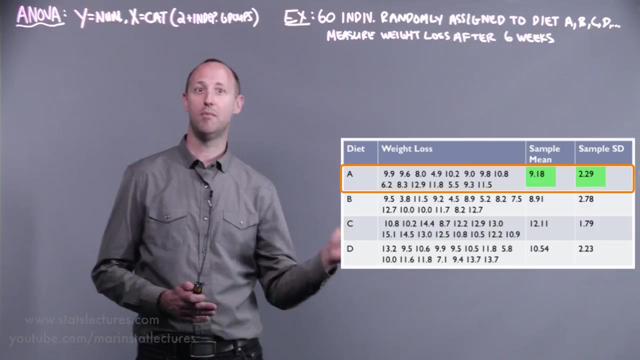 And we can see all the observations for group A here. They have a sample mean of 9.18.. Pounds lost on average And a sample standard deviation of 2.29.. Again, on average, an individual within diet A moved about 2.29 pounds from the mean of 9.18. 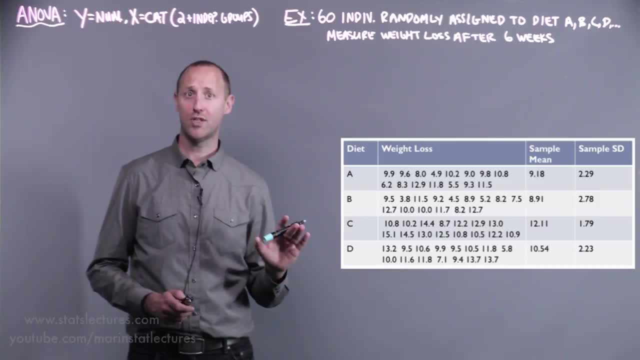 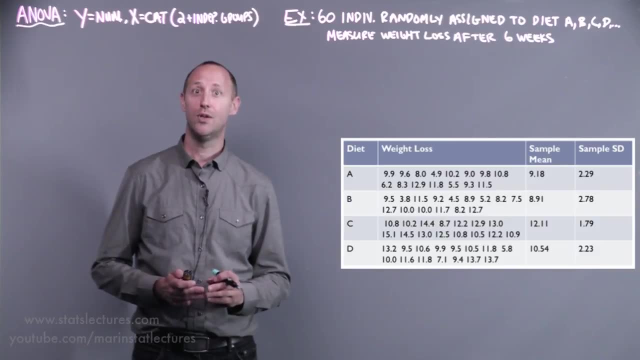 So we're going to work with simple data again to be able to focus on the concepts and not get overwhelmed with an extremely large data set. So what we'd like to do is we'd like to test: do any of these diets have an effect on weight loss? 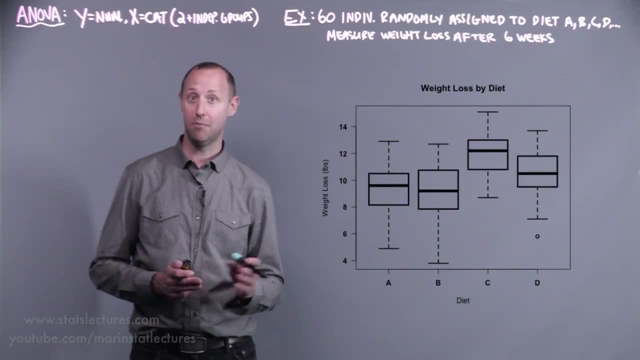 To try and get at that question, we can think of a simple data set that we can use to test weight loss. We can think about comparing the mean weight loss for each of the four groups or comparing the median weight loss for all the four groups. 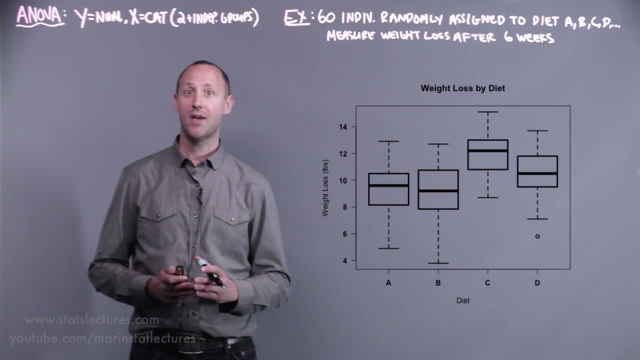 We're going to stick to comparing means and mention that if we want to compare medians, we can use non-parametric approaches or other approaches, bootstrapping or resampling approaches being one of those. So to try and get at this question, we're going to start with a null hypothesis. 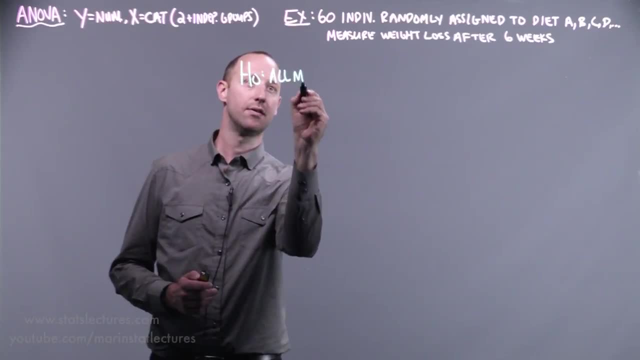 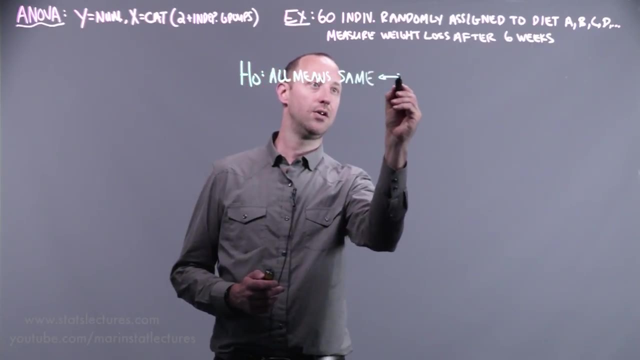 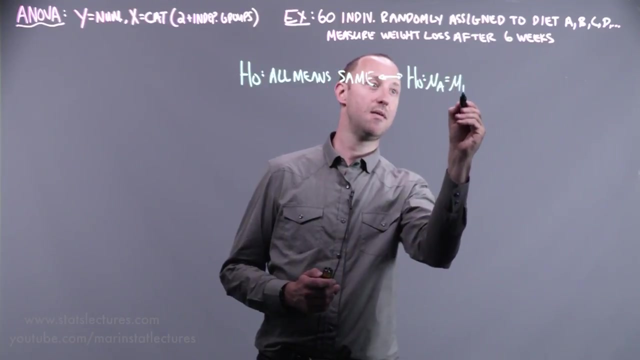 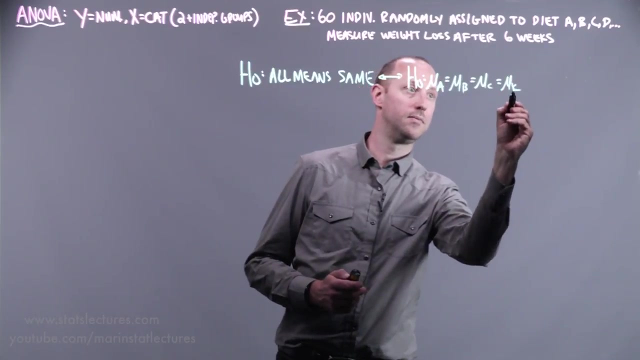 that all of the means, the mean weight loss in all these four groups are the same. we're expressing it in notation: The mean weight loss for someone on diet A is the same as the mean weight loss for diet B, the same for C and the same for D. 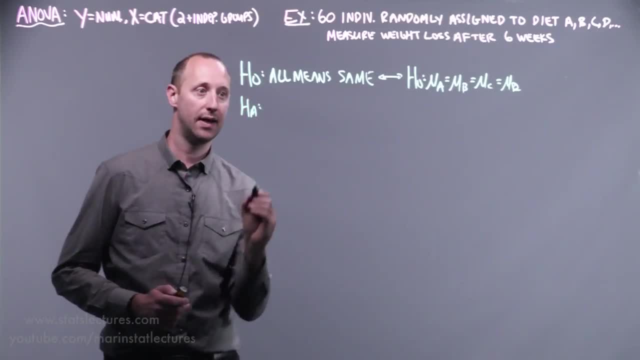 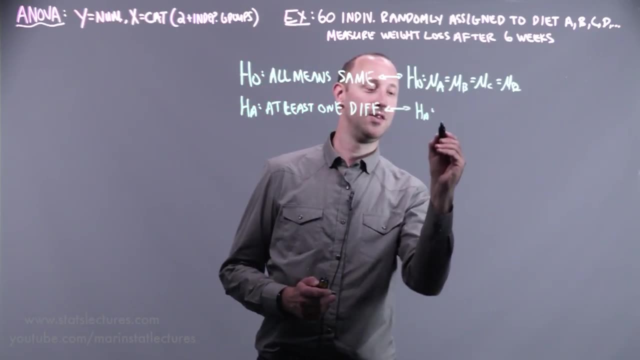 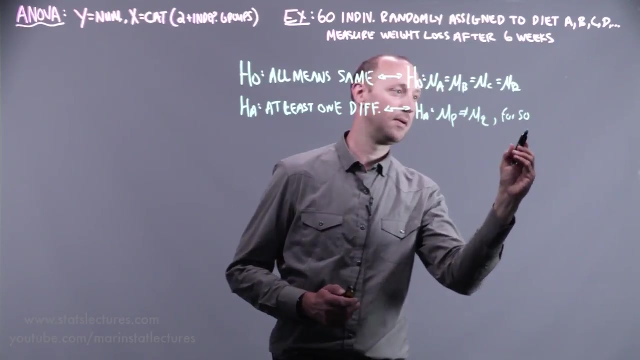 And an alternative hypothesis that at least one differs. And again, sometimes this is written: the mean weight loss for someone on diet A is the same as the mean weight loss for diet B and the same for D. The mean for group P is not equal to the mean for group Q. for some, P not equal to Q. 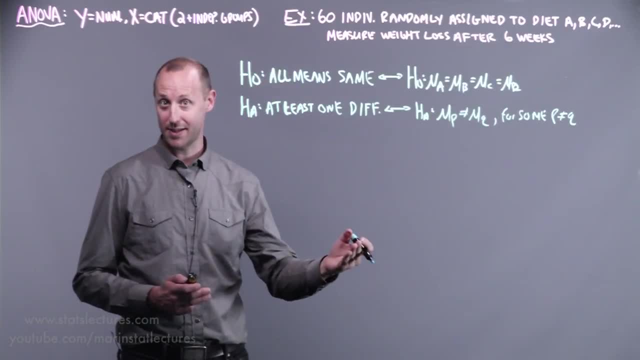 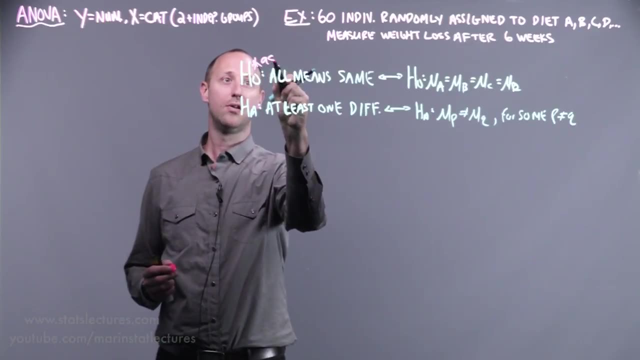 And again, this is just a notation-y way of saying at least one of the diets is different than the others in terms of mean weight loss. So a reminder: we start by assuming our null hypothesis to be true. Most hypothesis tests work this way. 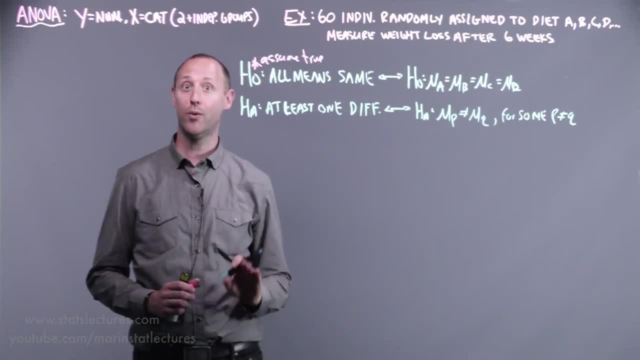 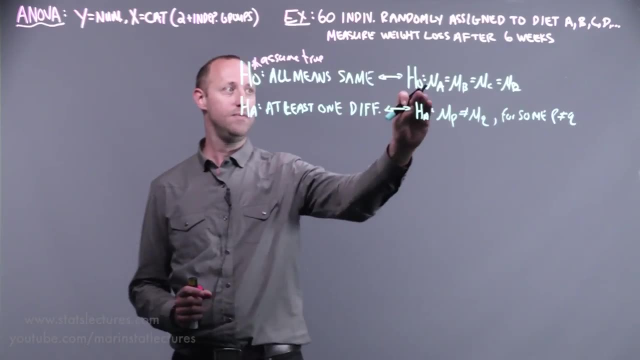 And again, that's because if the null is true, we know what we expect to show up in data. If, at the population level, the mean weight loss is the same for all these diets, we expect the sample means for all these four groups to be approximately the same. 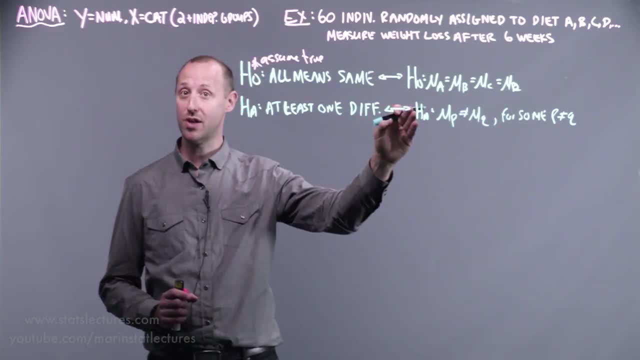 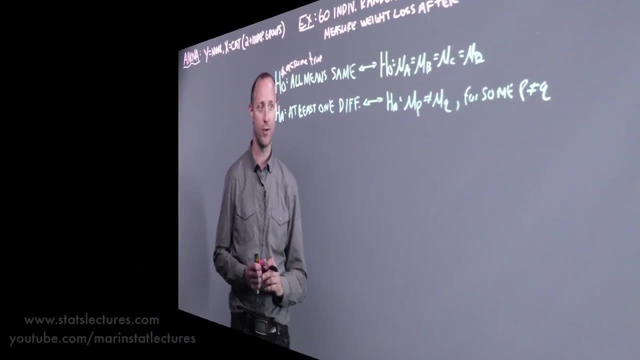 And then we can test how likely we were to see the differences we saw, or even larger if we'd expect them to be all the same. So hypothesis tests always have the same underlying approach. I like to think of ANOVA as sort of being a screening test. 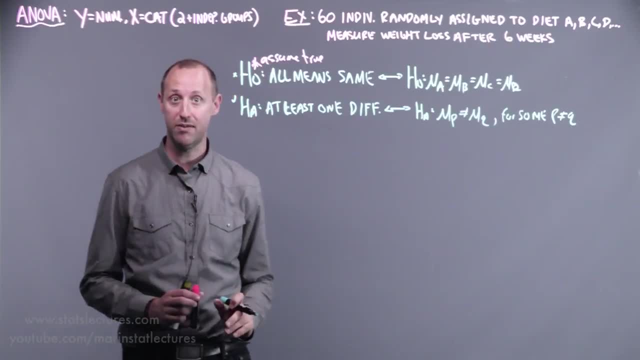 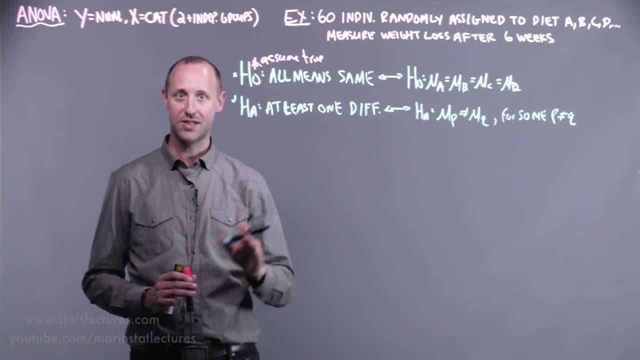 If we end up rejecting it, we're not going to be able to do it. Rejecting our null and saying we have evidence to believe the alternative is true. That just tells us at least one diet is different from the others. Here, at least one mean is different from the rest. 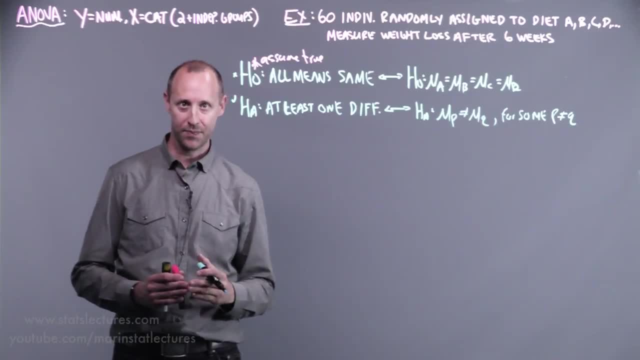 It doesn't tell us if more than one differ or which ones differ, and at that point We'll go in and we'll start to try and decide which diets differ from each other. Okay, which groups differ from each other? so we'll build our way up to that. so, before getting into the mechanics of the test, 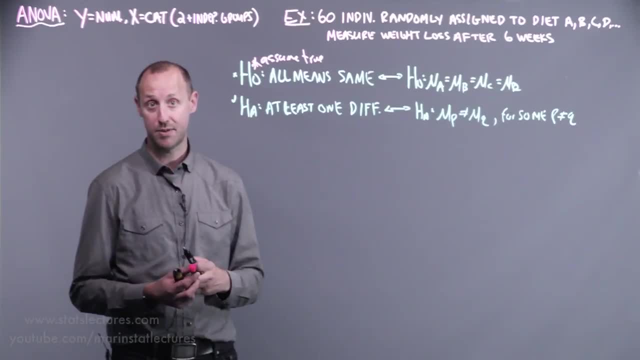 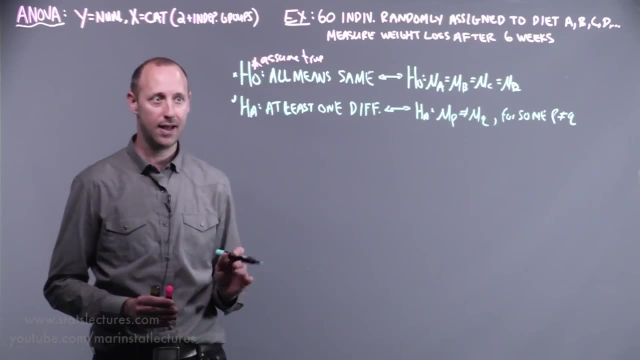 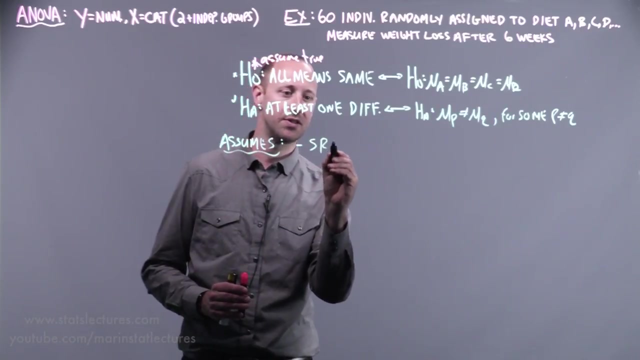 Let's just spend a moment talking about The assumptions of this right. so again, This is another parametric approach, or sometimes called large sample approaches, and it has the same general set of assumptions To work with one-way analysis of variance. We're going to assume we have a simple random sample. 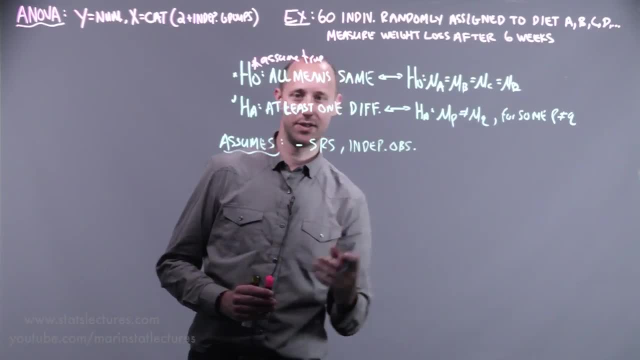 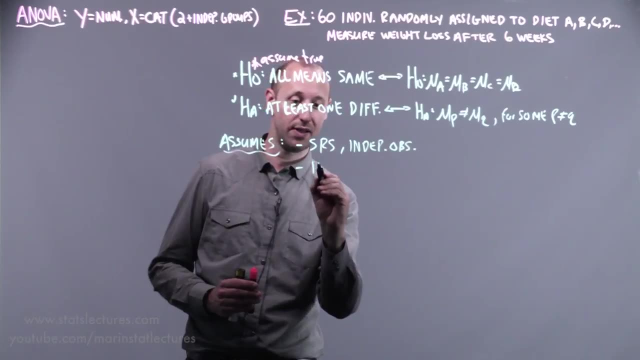 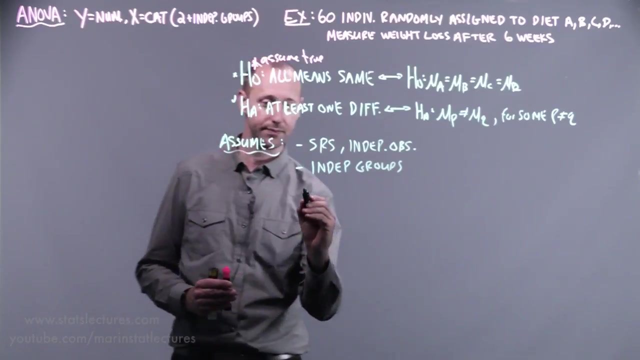 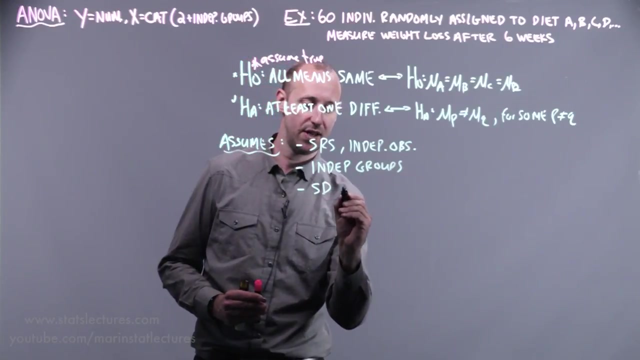 We have independent Observations. so person one, person two, person three, They're all independent of each other. We're going to Assume that we also have independent groups. So in this example, people on diet a are independent of the people on diet B. We have the equal standard deviations assumption, so we assume that the standard deviation of each group 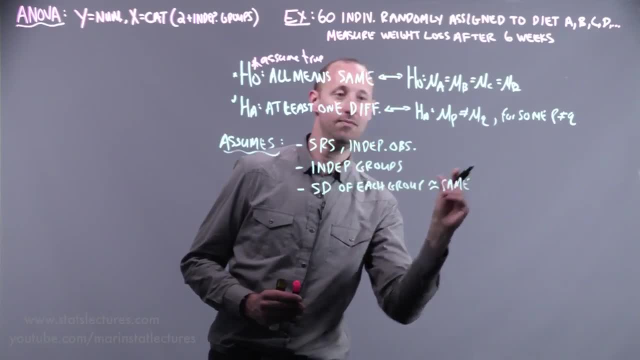 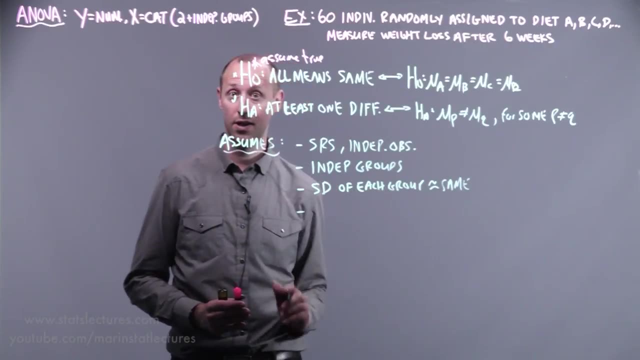 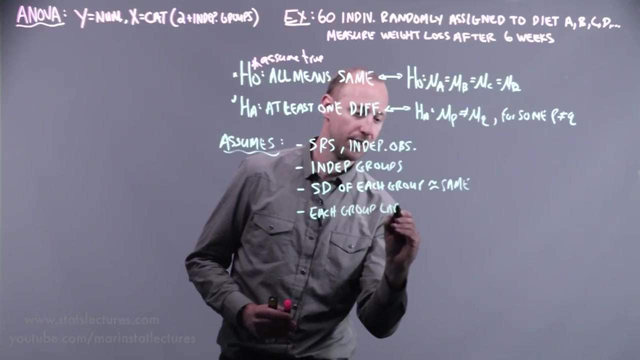 Is roughly the same. Again, at the population level, the variability and weight loss under these four diets is approximately the same. and then, finally, the large Sample assumption. We assume that each group Has a large Sample size, Bigger than 20, as the guide right. we've noted before that. 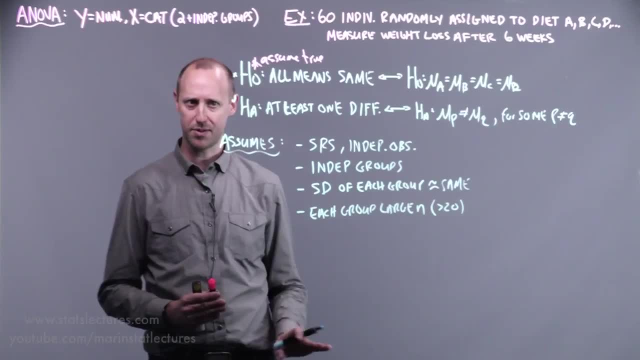 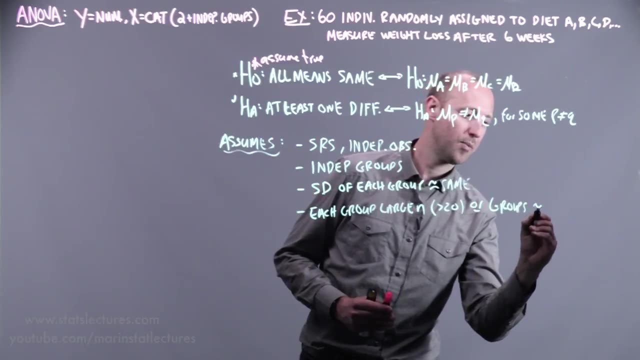 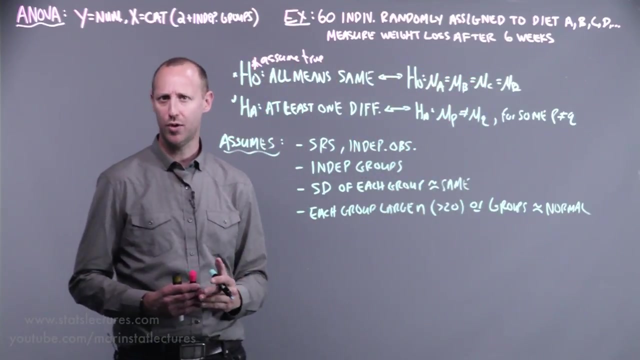 the more skewed each group is, the larger the sample size should be. so 20 is just a rough guide. or groups are Approximately normal. So the distribution of weight loss in each of these four groups Is approximately normal or symmetrically distributed around its mean, as we've hit on in other videos. 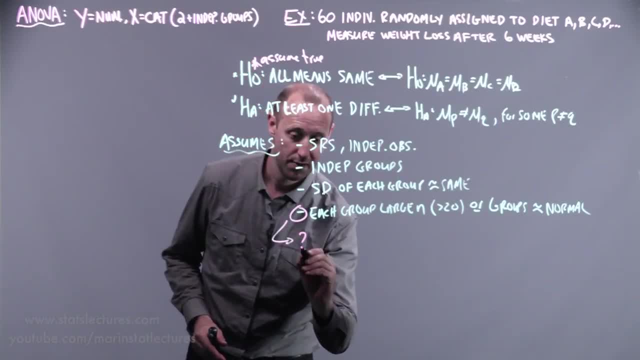 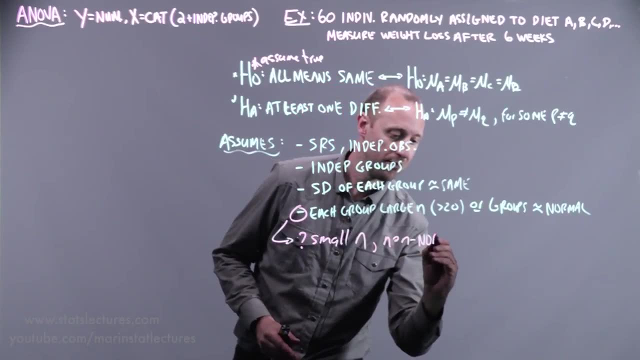 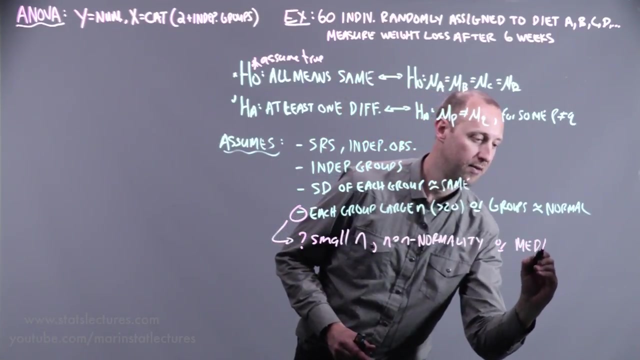 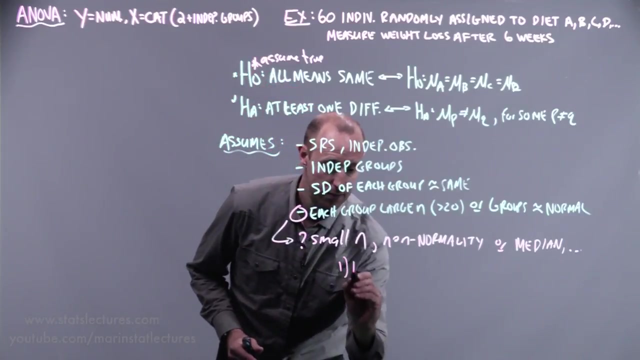 What if these assumptions aren't met? What if we have a small sample size, We have non normality, Or What if we want to test about median rather than means? Then we can use either non parametric approaches Or non parametric approaches, So we can use a. 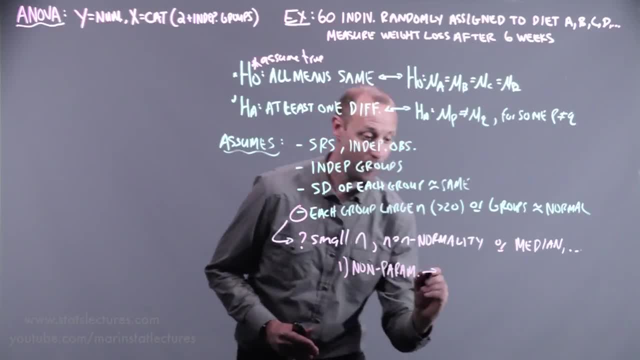 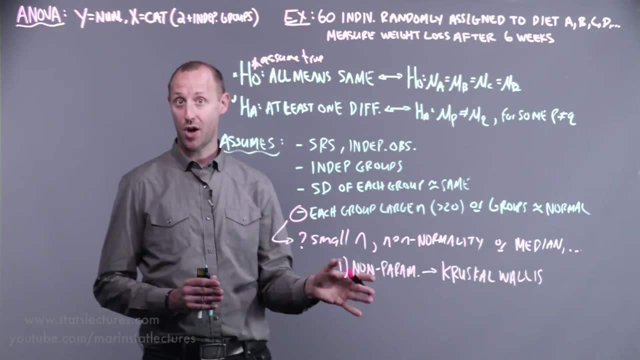 non-parametric approach, and The one in this case would be the Kruskal-Wallis. We can use Kruskal-Wallis one-way analysis of variance. So this is the non parametric alternative to one-way analysis of variance. works pretty similar to the tests. 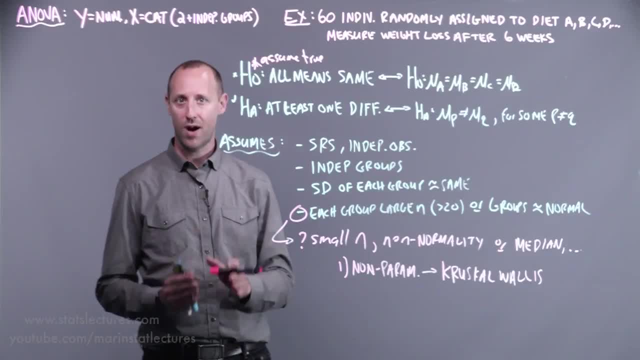 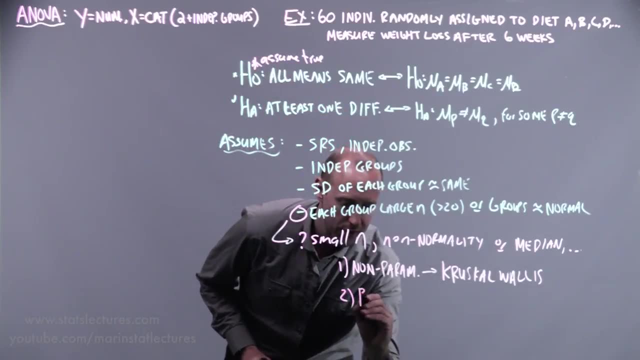 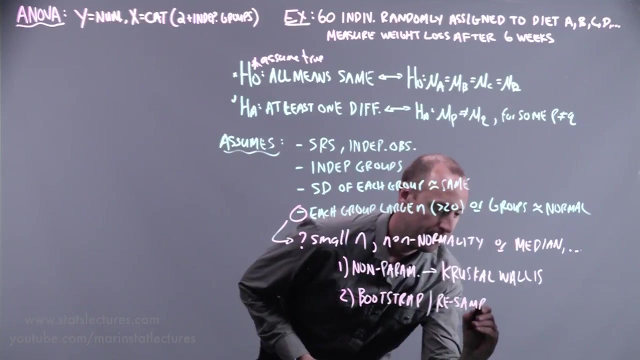 We've the non parametric tests we've seen so far. Rather than using actual values, it ranks them and then it compares the ranks in some way. or We could also consider using some form of bootstrap or a resample Type approach, and we've touched on these to some extent and laid 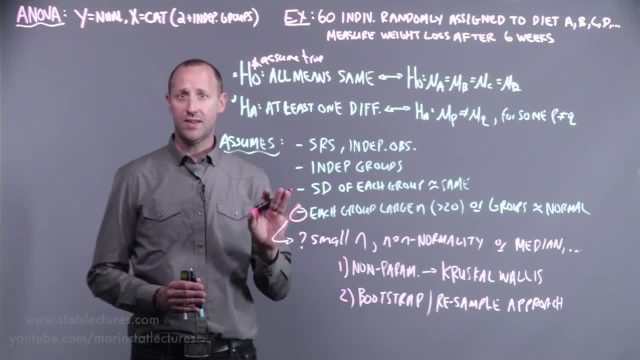 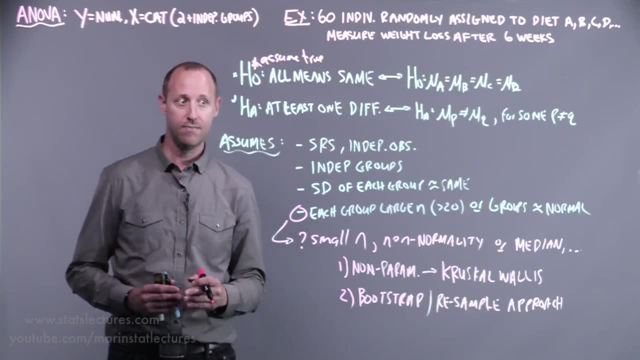 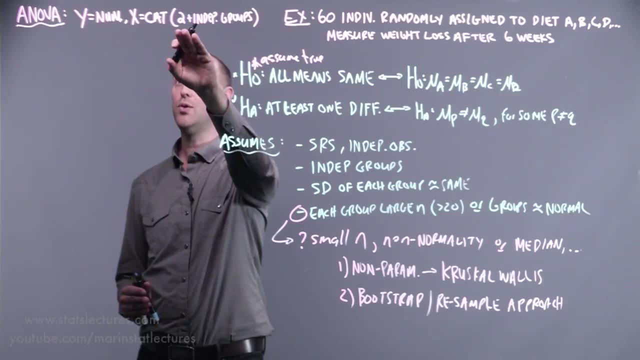 foundation for these to some extent. so we can think of the Analysis- one-way analysis- of variance as being an extension of the independent two sample t-test Has all the same set of assumptions. it's just for testing The comparing the means of two or more independent groups in the case that we compare two independent groups.